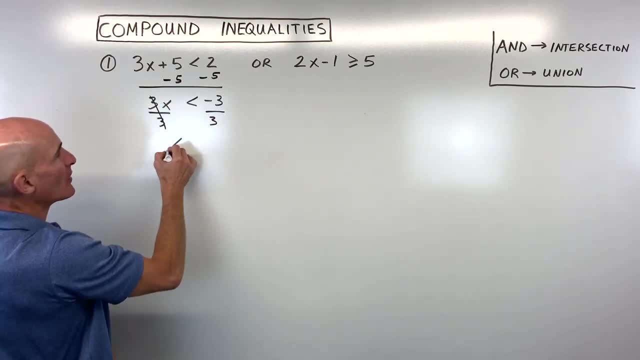 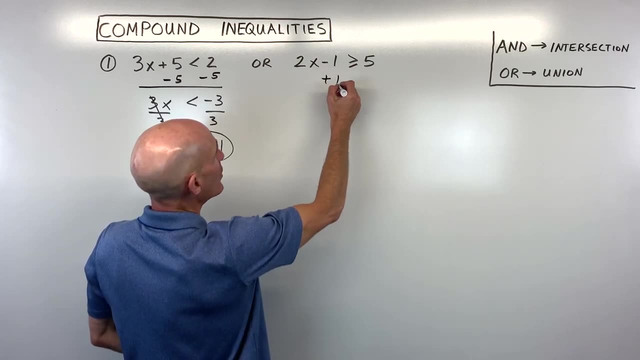 both sides by 3 to get x by itself. So now we have: x is less than negative 1.. And then over here we're going to try to get this variable by itself. So first we're going to add 1 to both sides. 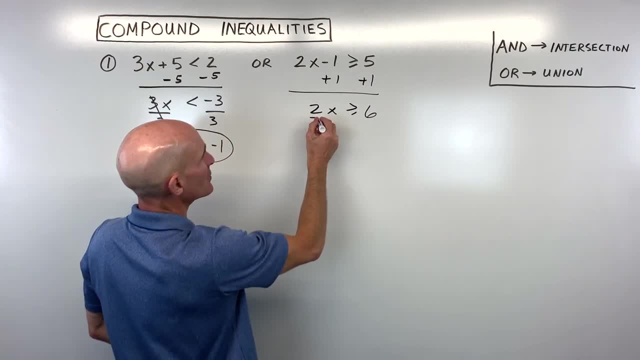 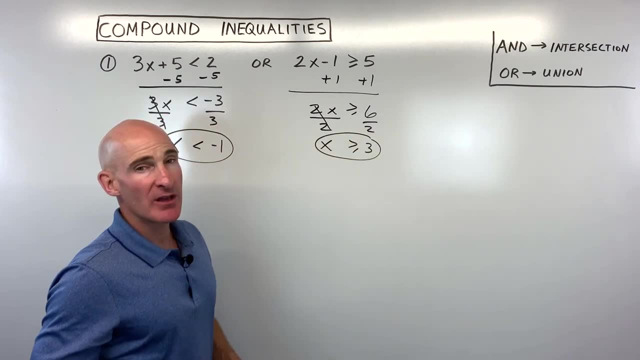 So we have: 2x is greater than or equal to 6.. And then we're going to divide both sides by 2. And we can see that x is greater than or equal to 3.. Now, one thing you want to be careful of when you're solving inequalities is that if you multiply or divide by a negative 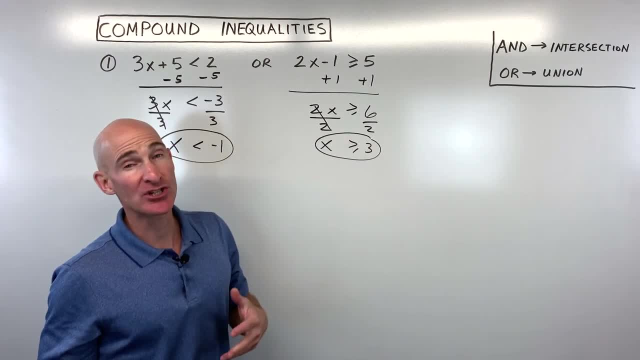 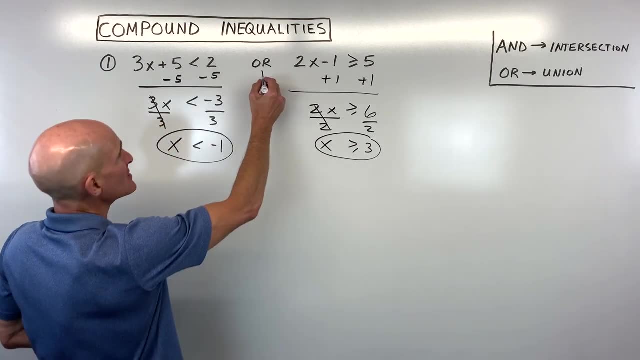 number. what happens is the inequality sign is going to flip or change direction. So just if you yourself multiply or divide both sides by a negative number- Now notice this is an or. So what we can do is we can go to our number line and we can say: x is less than negative 1.. 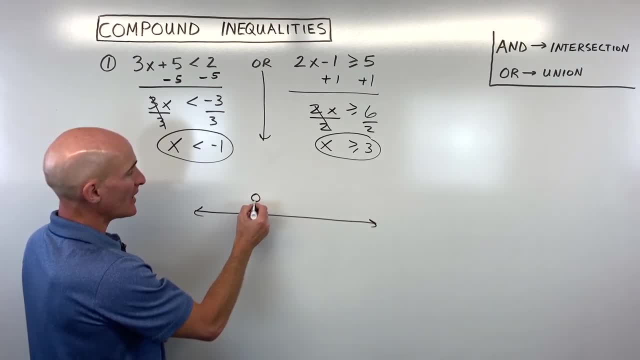 So what does that mean? less than negative 1?? Well, it doesn't include negative 1.. So we're going to draw this as an open circle like hollow. Less than means it includes the points here that are less than, or lower or smaller than negative 1.. 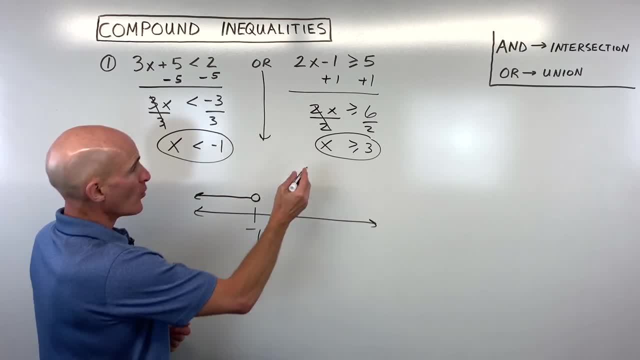 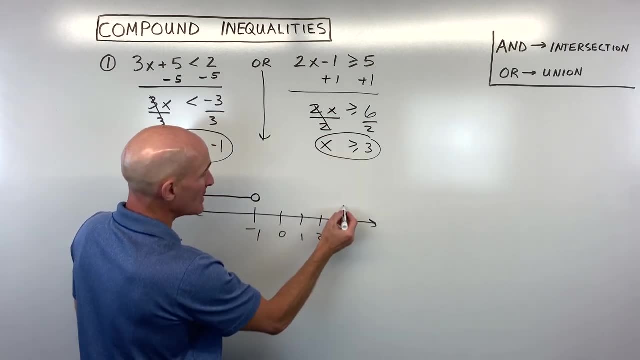 And as we go to the left, the numbers are getting smaller right. Whereas the second inequality, let's go over to 0,, 1,, 2,, 3.. x is greater than or equal to 3.. So equal to 3. 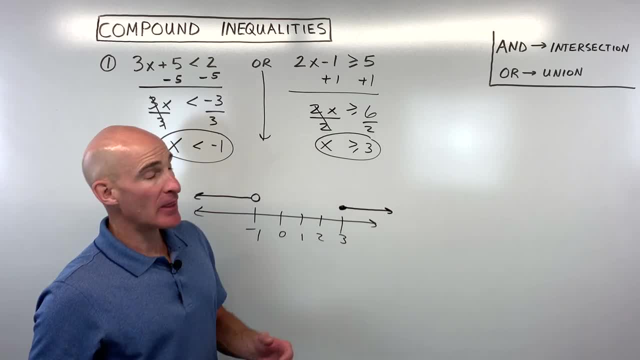 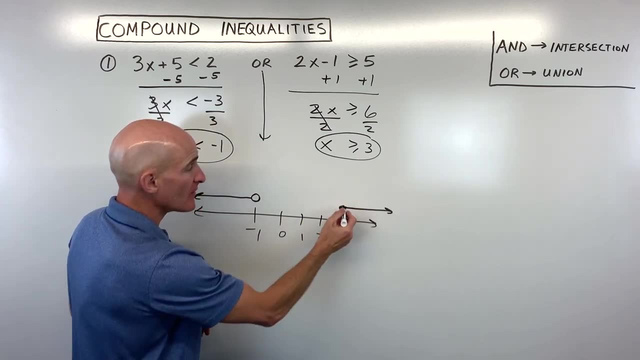 or greater. As we go to the right, the numbers are getting larger, And then when you see that word or that means union, It means it's all of these values as well as all these values, So it's like the combination of the total here. So it's basically everything that we have graphed. 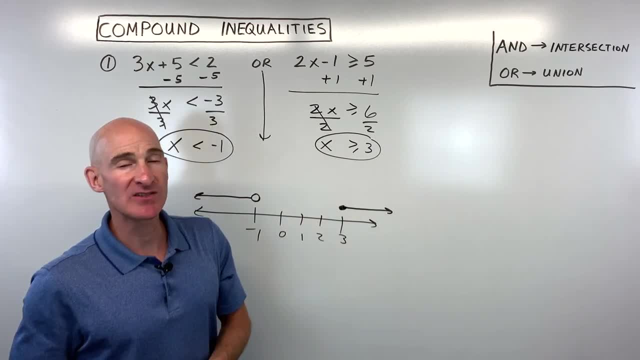 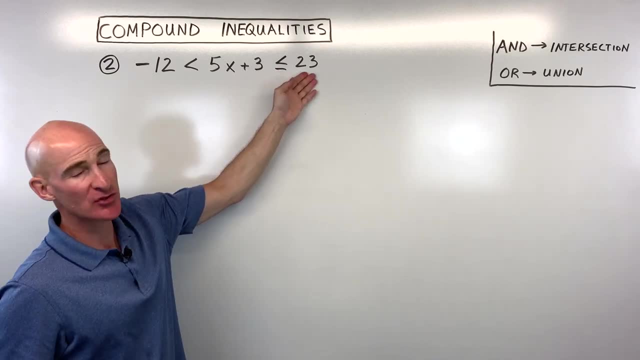 So this is the solution to the first example. Let's take a look at the next example. okay, let's look at number 2. now we've got negative. 12 is less than 5x plus 3 is less than or equal to 23.. 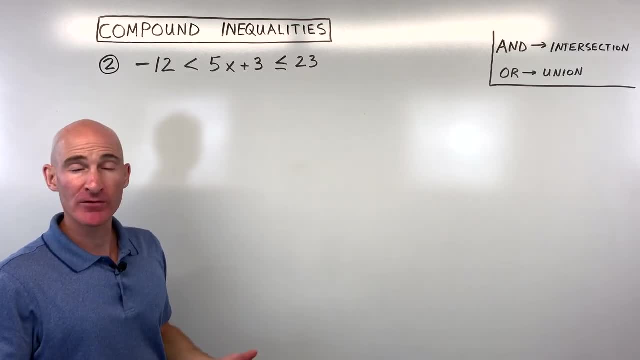 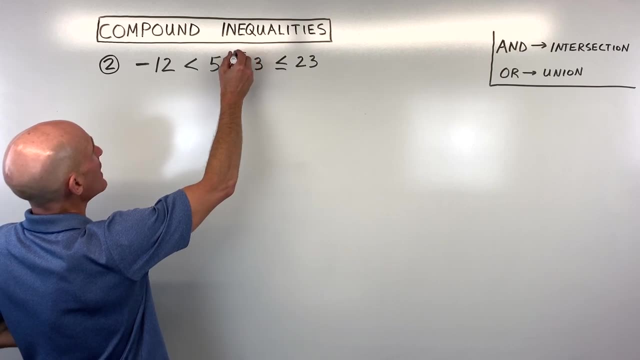 So this particular one is different than the first example. The first example was an or. This one is an implied and. And what does that mean? Well, you can see. what we have here is we have actually 2 and 1.. inequalities that are put together. We have this one, which- let's write it over. 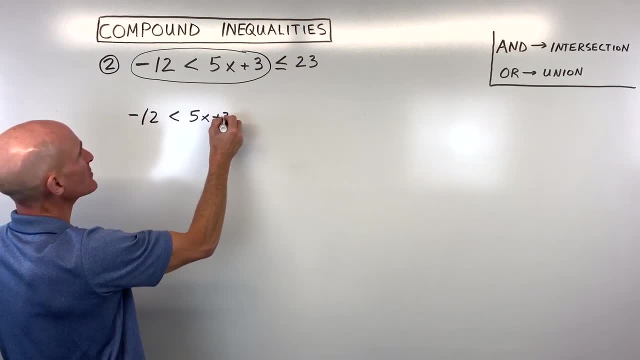 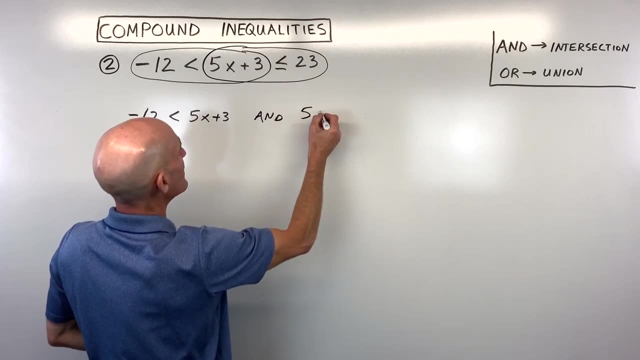 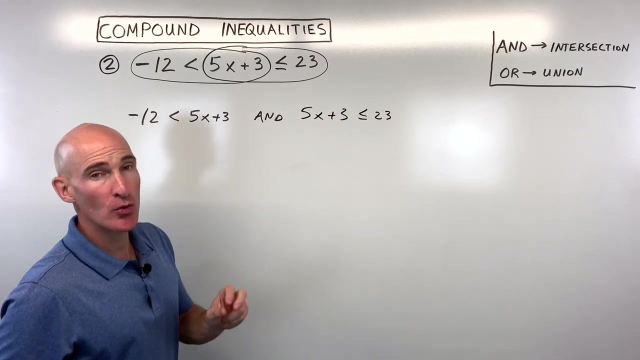 here separately. Negative 12 is less than 5x plus 3.. And here's our implied- and We have this inequality on the right side We have 5x plus 3 is less than or equal to 23.. So one way to do this is to split it apart into two inequalities and solve. 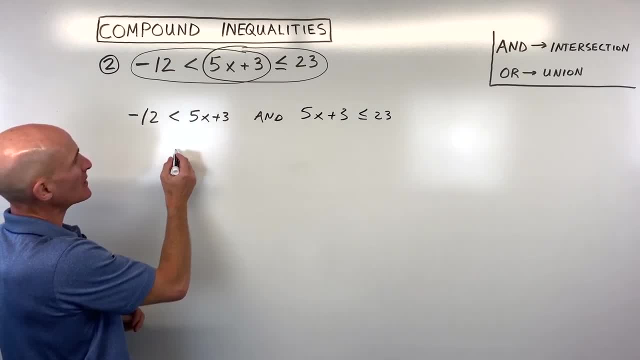 them separately. So let's go ahead and do that. So what we're going to do is think about getting the variables on one side, numbers on the other. So I'm going to subtract 3 from both sides of the inequality And we want to solve for x. 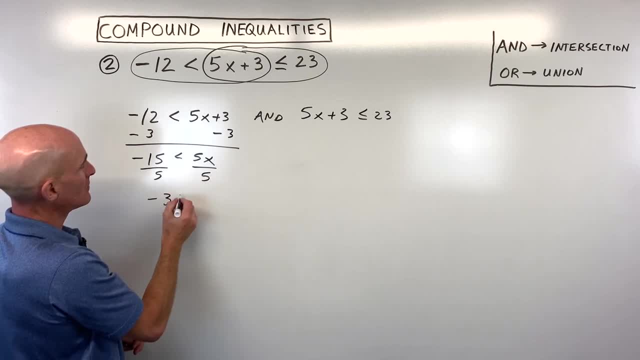 I'm going to divide both sides by 5.. Okay, And so now we have: negative 3 is less than x. Or you could say x is greater than negative 3.. I just flipped that inequality over. For the second one, we're going to get the numbers on one side. 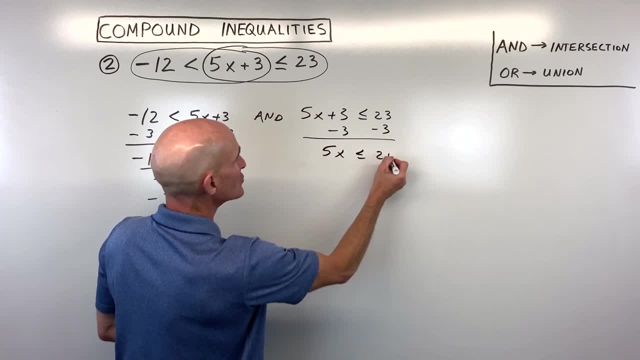 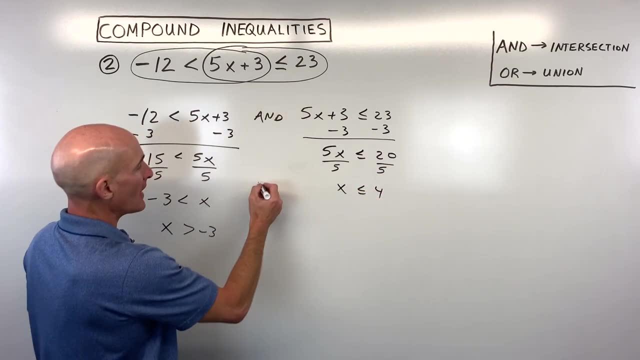 variables on the other. So we have 5x is less than or equal to 20.. Divide both sides by 5 to get x by itself, So we have x is less than or equal to 4.. And keep in mind that this is an, and So our. 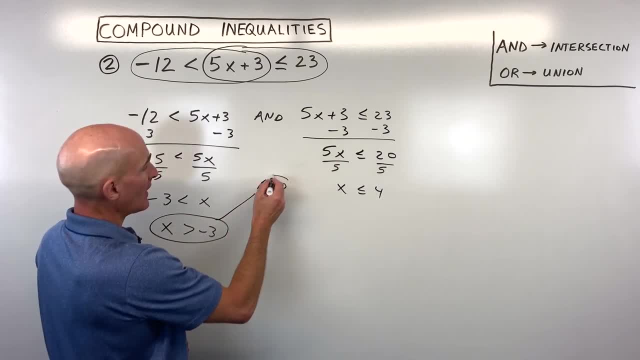 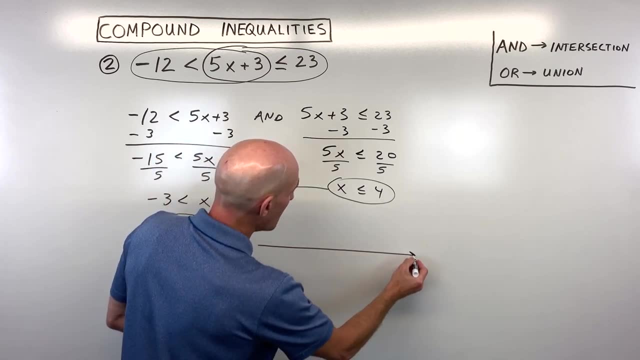 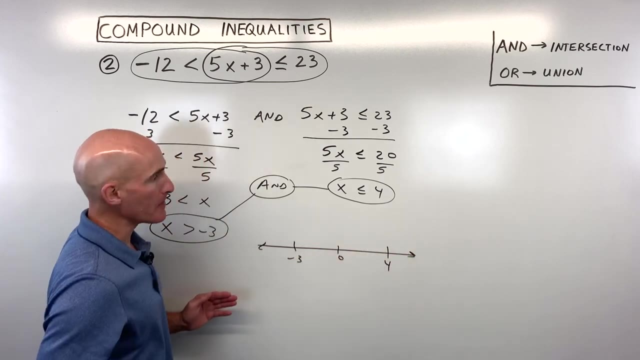 solution is: x is greater than negative 3 and x is less than or equal to 4.. Now, graphically, what this looks like. on the number line, negative 3 is over here, 0 is somewhere over here, 4 is somewhere over here. I'm going to go from low to high. So what we have is x is. 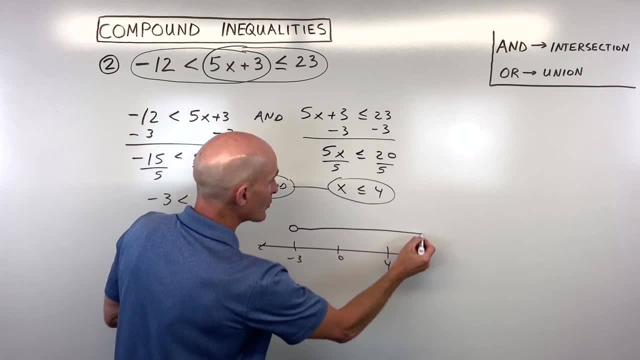 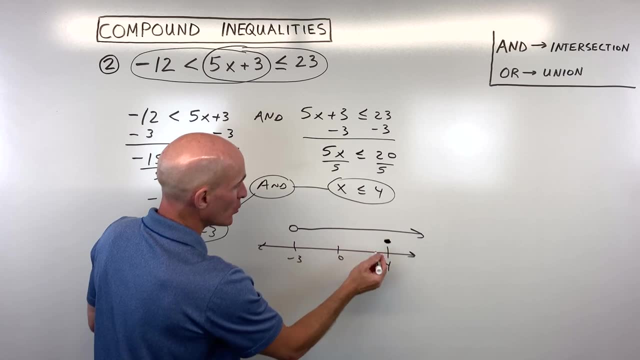 greater than negative 3. So greater than. we're graphing to the right, It's getting a lot larger And at the same time x is less than or equal to. So equal to is a closed circle. Less than means we're going to the left, or smaller. But the and means the. 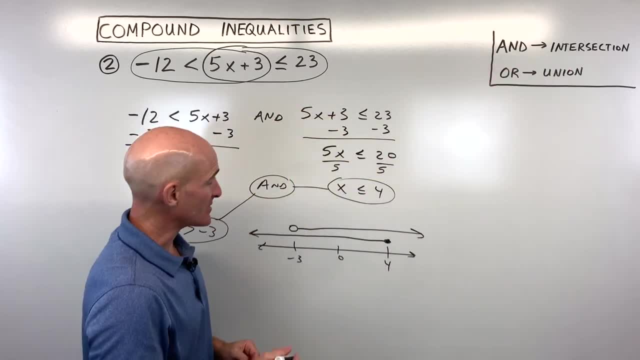 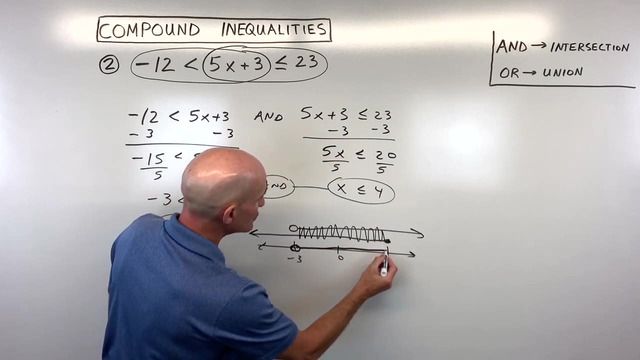 overlap or the intersection of the two sets. It's what they have in common. So you can see they're overlapping right here. Okay, Up to that point. So our final result, our answer here that we can graph on the number line, is going to be from negative 3 to 4,. 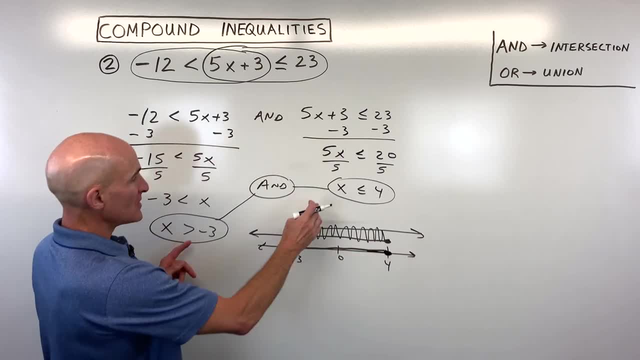 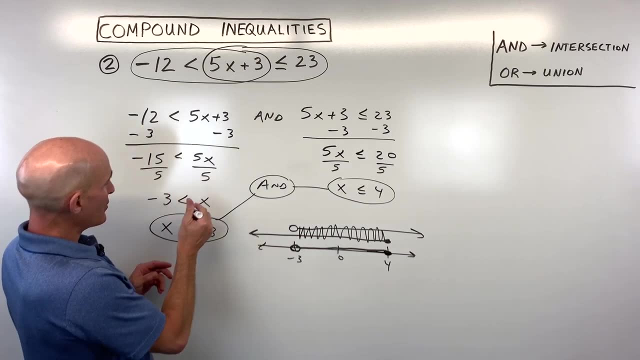 including 4.. And what we can do with these two inequalities? we can put them back together as like one inequality. And the way that I would do that is: you see here how we have: x is greater than negative 3, or negative 3 is less than x. So let's write that down: Negative 3 is less. 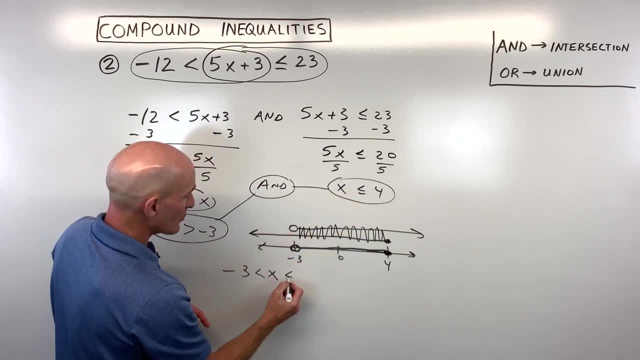 than x And at the same time, x is less than or equal to 4.. And so you can see, x is in between- see negative 3- and 4.. Not including negative 3, but including positive 4.. It's. 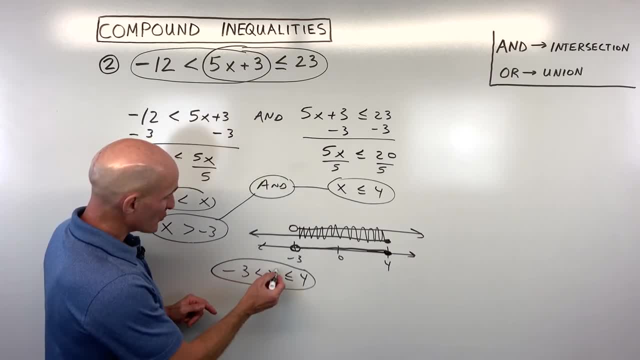 like x is sampled, It's like x is sandwiched in between, And you can still see we have those two inequalities here. We have x is greater than negative 3 and we have x is less than or equal to 4.. It's just we put them together as like one inequality. But one thing: you want to be careful. 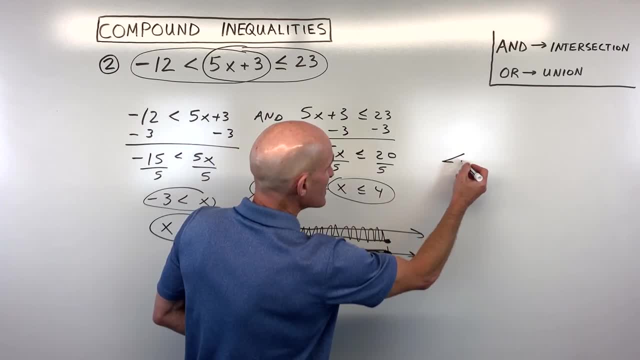 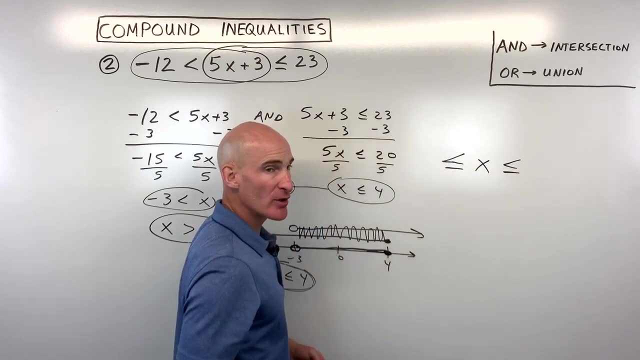 of when you put these together. you always want these inequality signs to be pointing to the left, So they could be less than or less than or equal to. You always want that variable in the middle And you're going to find that the smaller number here is on the. 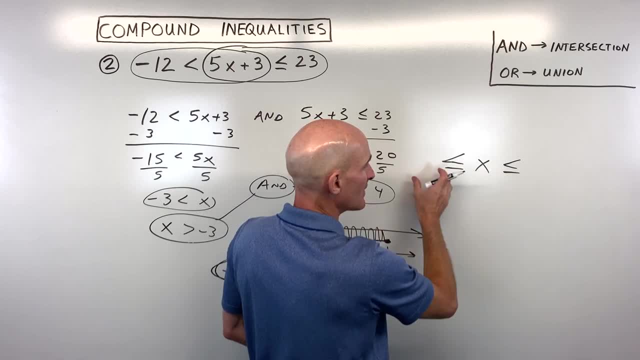 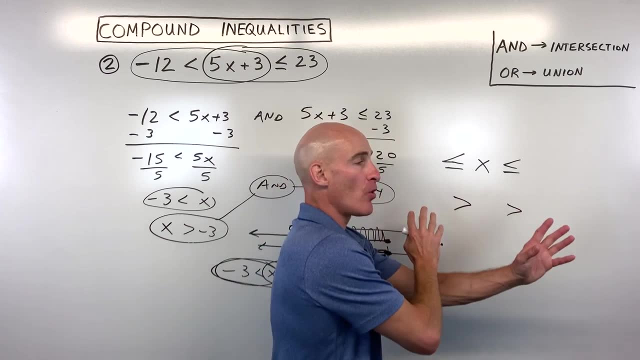 left. The smaller number is here on the right And the variable is like in between that smaller and greater number. Now if you have a situation where they're pointed like this, you can flip this whole inequality so that it's in this proper form. Let's take a look at another. 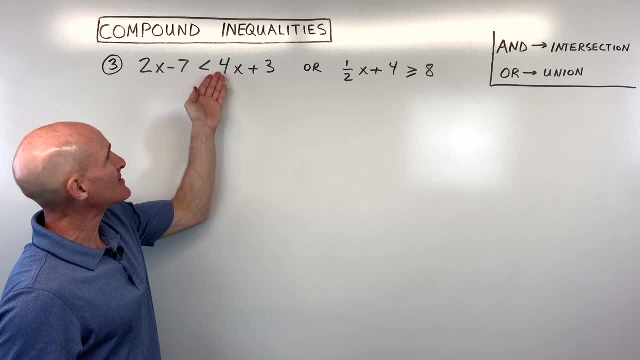 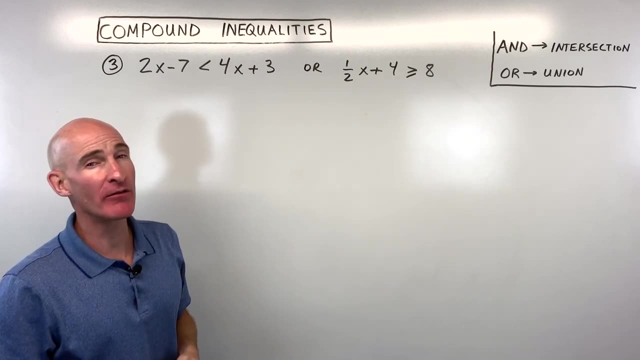 example For number 3, we've got: 2x minus 7 is less than 4x plus 3, or 1 half x plus 4 is greater than or equal to 8.. So how would we solve that one? Well, when it's an or, we can just: 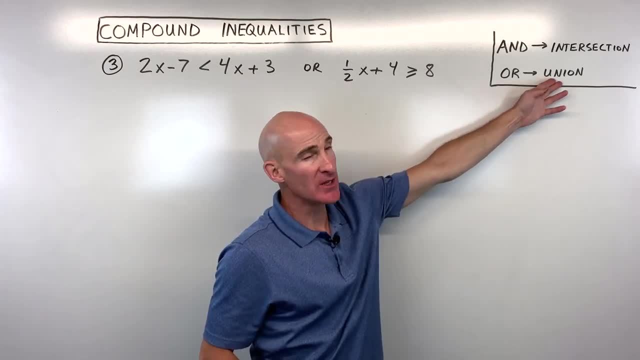 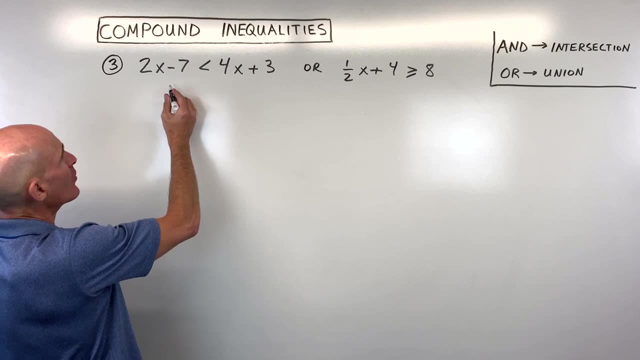 solve these individually And then remember, or means union. So it's like we're going to look at the combination of the two solution sets. So when we do this, we want to get the variables on one side, numbers on the other, just like. 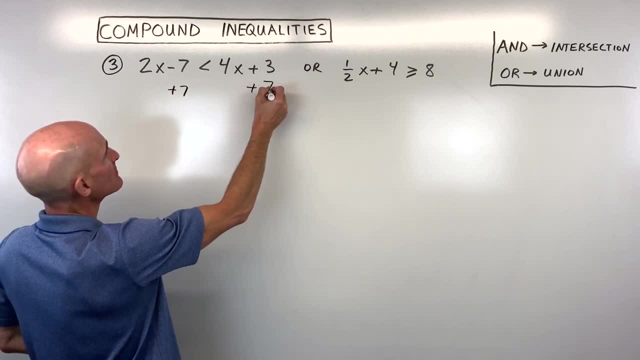 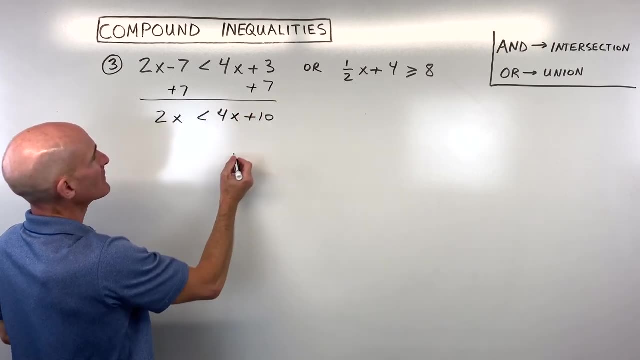 solving equations. So what I'm going to do is I'm going to add 7 to both sides. Okay, so that gives us: 2x is less than 4x plus 10.. Then I'm going to get the variables on the. 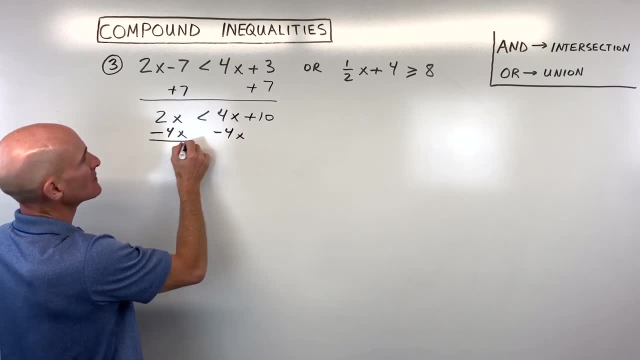 other side. So I'm going to subtract 4x from both sides, So that gives us negative 2x is less than 10.. And then I'm going to divide both sides by negative 2 to get x by itself. Now remember, when you multiply or divide both sides by a negative, the inequality sign. 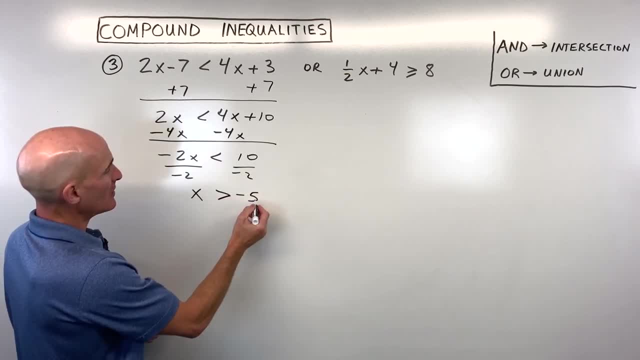 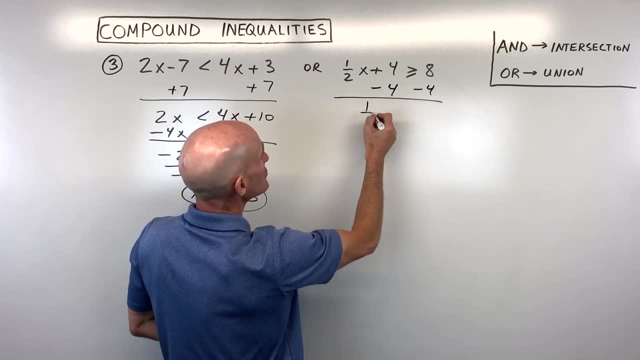 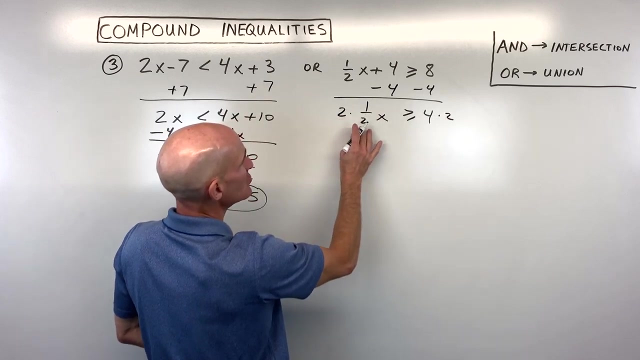 changes direction. So this is going to be: x is greater than negative 5.. Now for the other inequality. we're going to get the variables on one side, numbers on the other. So we have 1 half x is greater than or equal to 4.. Let's multiply both sides by 2, because 1 half times. 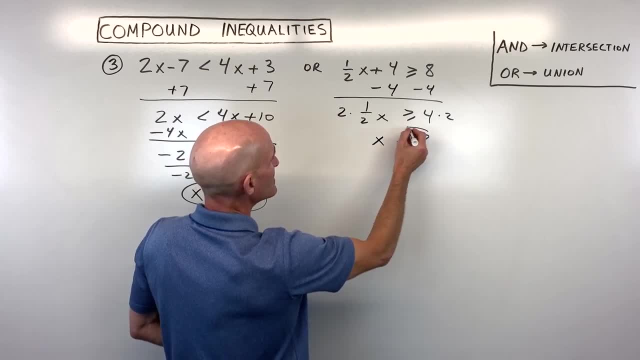 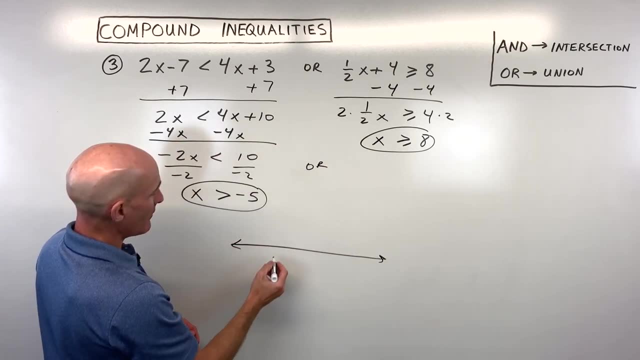 2 is 1.. That'll give us the variable. by itself, x is greater than or equal to 8.. Okay, so we have. let's go to the number line. Now we've got these two inequalities, we have negative 5.. So x is greater than negative. 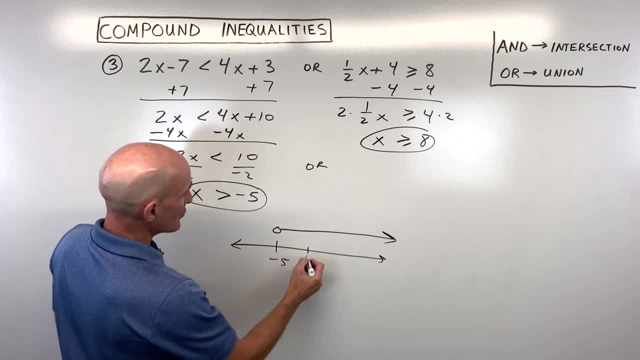 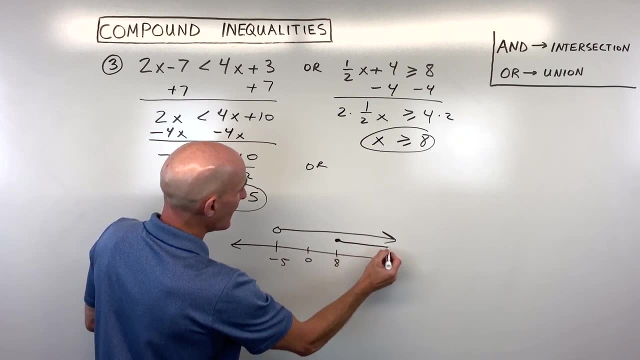 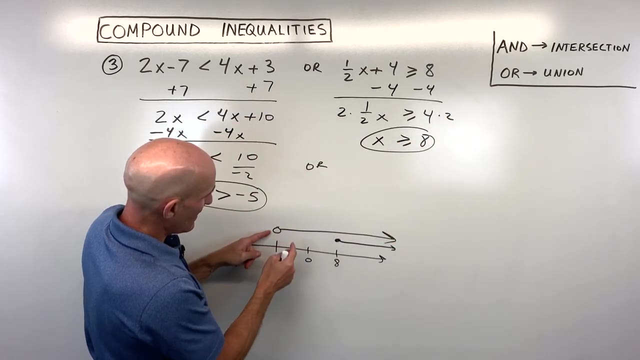 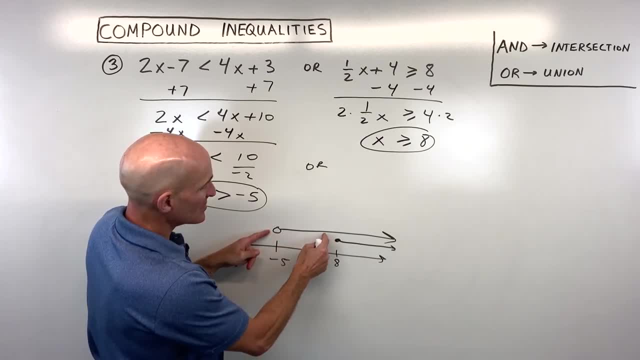 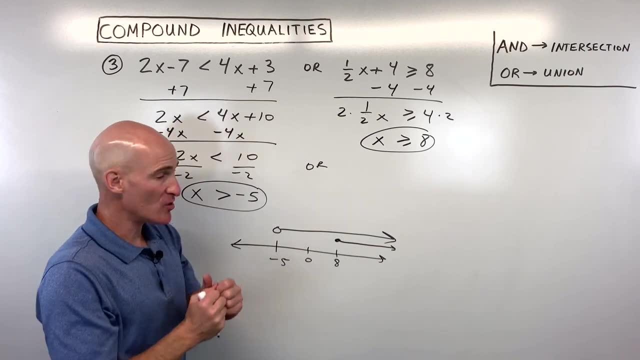 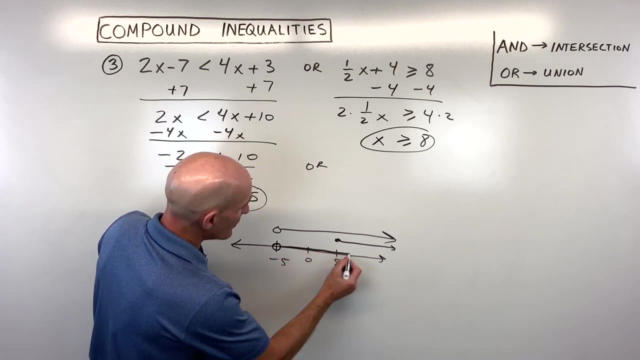 4.5, negative 4, all these numbers here, as well as all these numbers here. So we're like combining these together, It's the union. Union means like you're uniting the two sets. So our final result is going to be this, right here on our number line, And our answer is: 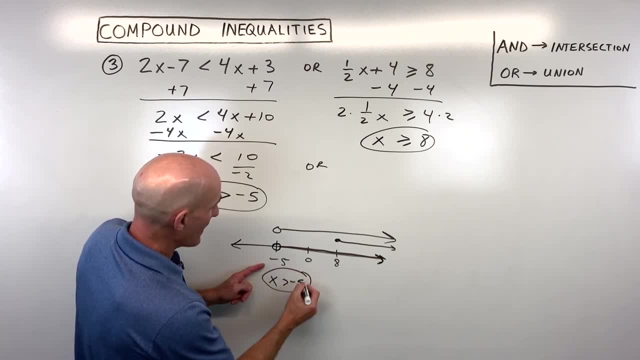 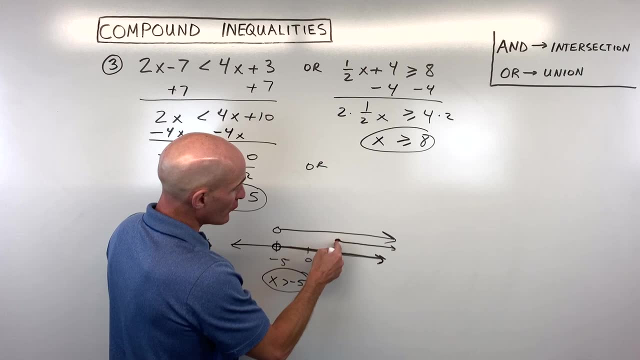 just going to be: x is greater than negative 5.. Now, if this was an and problem and means the intersection, we'd say: oh, where are they overlapping? They're only overlapping from 8 or to the right. So x is greater than or equal to 8.. But with or, we're talking. 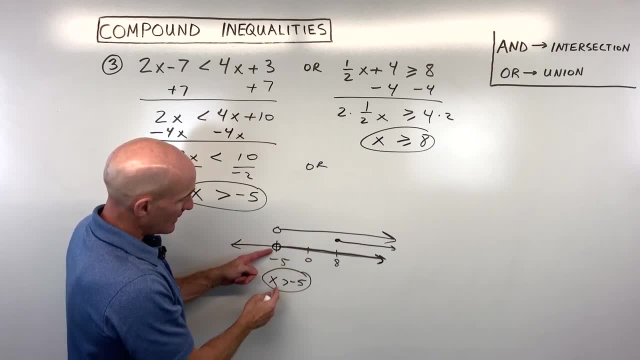 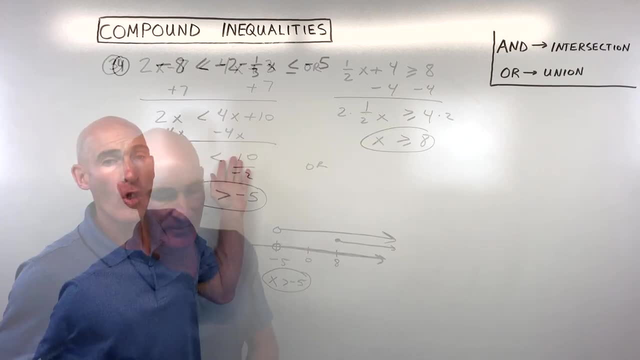 about union. we actually combine these together into 1, and that answer here is graphed on the number line x is greater than negative 5.. Let's take a look at another example. Okay, before we do this last number, 4 and type of. 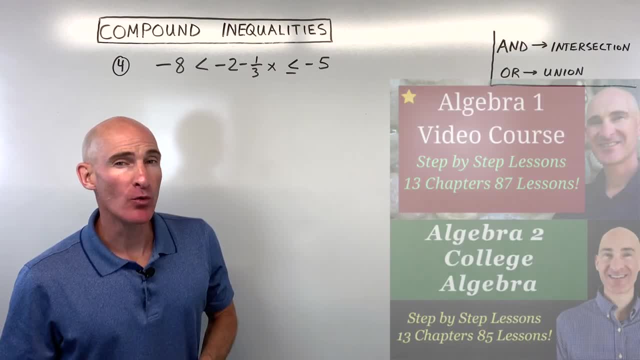 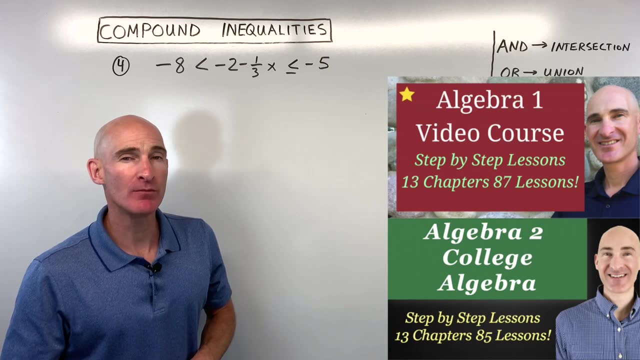 problem. if you like the way that I explain things and you want to go deeper into Algebra 1 or Algebra 2 with me, check out my video courses for sale. I'll put a link in the description below And I take you through. 85 lessons in the one course, 87 lessons in. 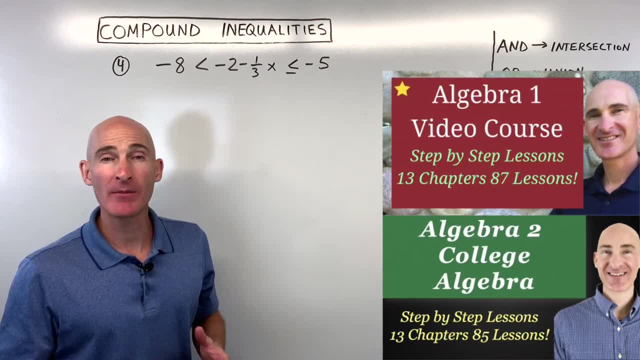 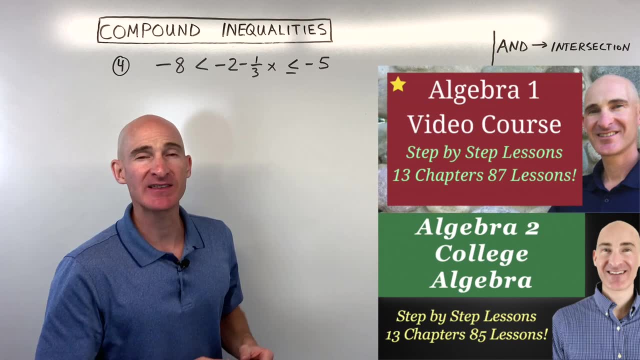 the other course. We go through the concepts, We go through example problems. I give you some problems that you can practice on your own and we'll go through those together as well, And I take you step by step, building on the previous concepts, to help you walk. 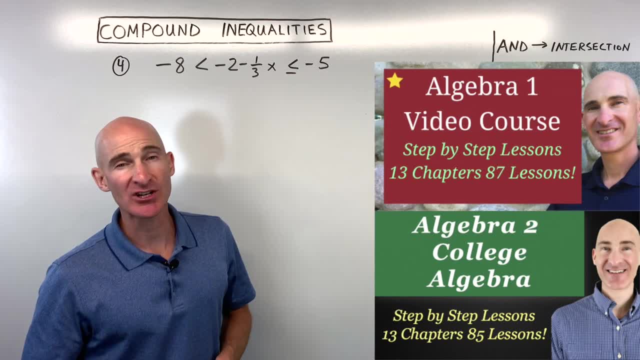 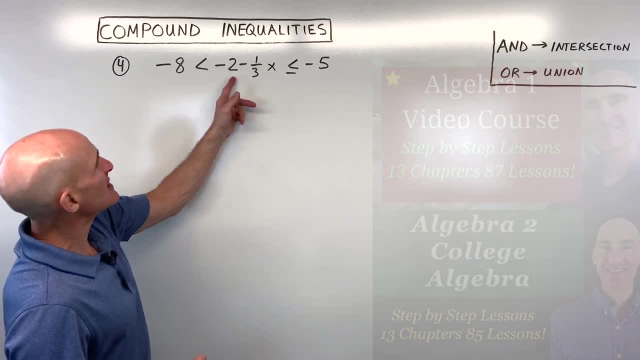 through both Algebra 1 or the Algebra 2 slash college Algebra course. So check those out if you're studying that, And let's dive into this last example together. So you can see that this is an and type, And in the first example we broke them apart into two separate inequalities and then at 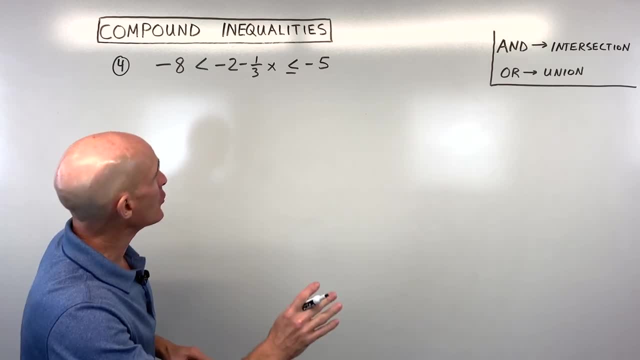 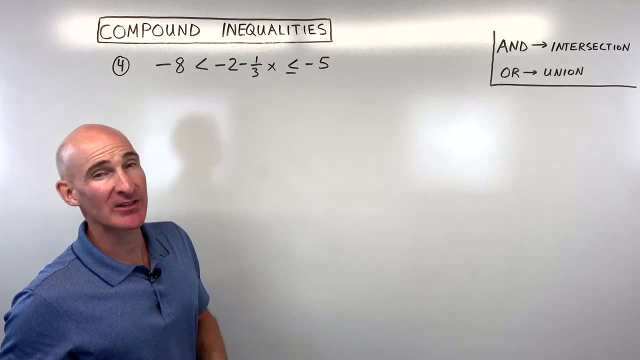 the very end we put them back together. Remember that. But there's another way to do this and that's to get the variable by itself in the middle, And it's like solving the two inequalities at the same time, like simultaneously. So what I mean by that is we're trying to get 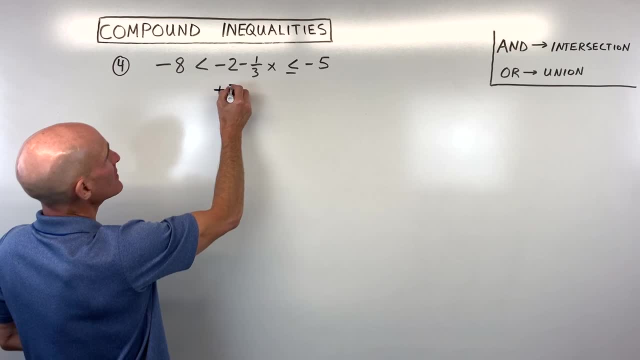 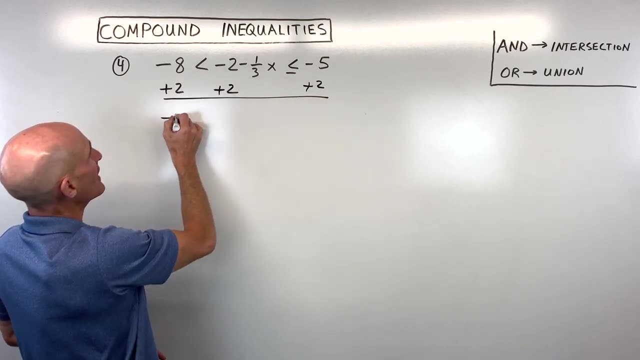 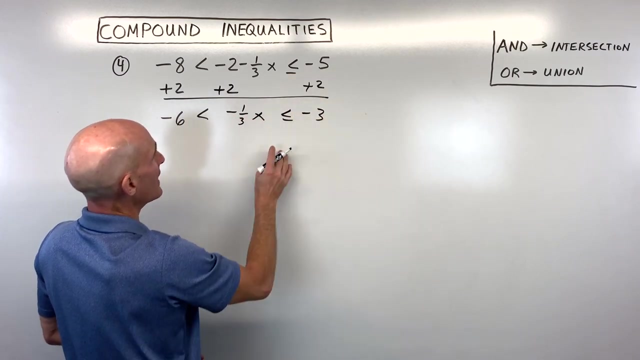 this x by itself. So instead of subtracting 2, let's add 2 to the left, to the right and to the middle, And so if we do that, you can see we're getting negative 6, which is less than negative one-third. x is less than or equal to negative 3.. Now here we want. 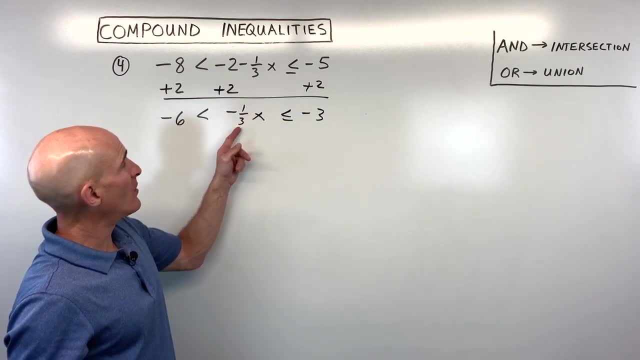 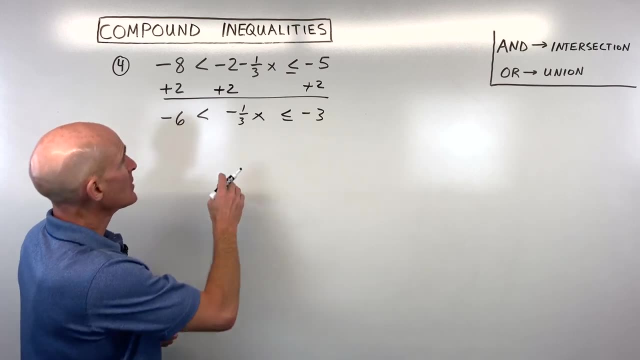 to get our x, our variable, by itself in the middle. So the negative one-third times x, we could divide by negative one-third or multiply everything by negative 3.. So let's go ahead and multiply by the reciprocal negative 3. That's going to give us 18 here. That's going. 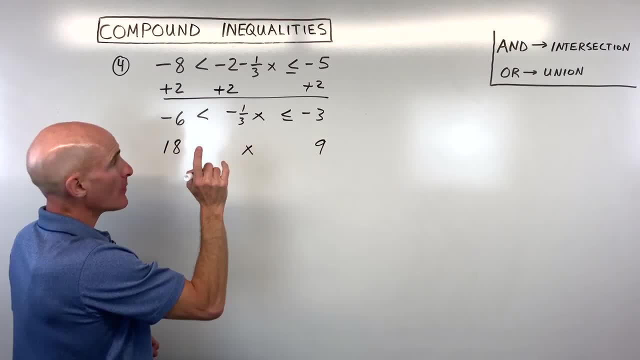 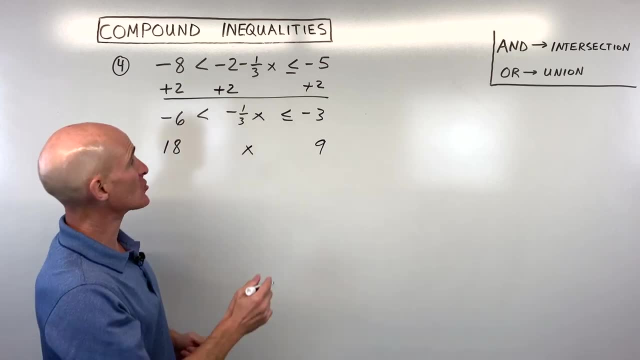 to give us 9 here. That's going to give us x here. But remember, when you multiply or divide both sides of an integral, you're going to get negative 3. So that's going to give you an inequality by a negative number. That inequality sign is going to change direction. 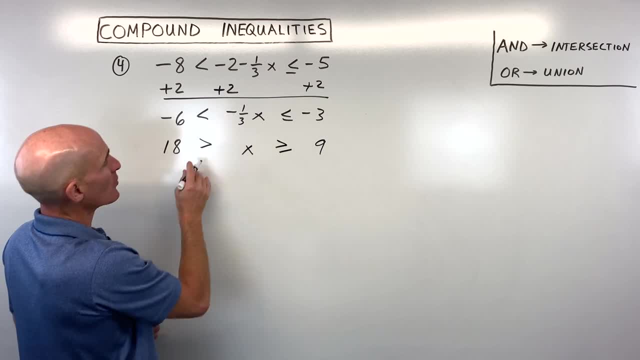 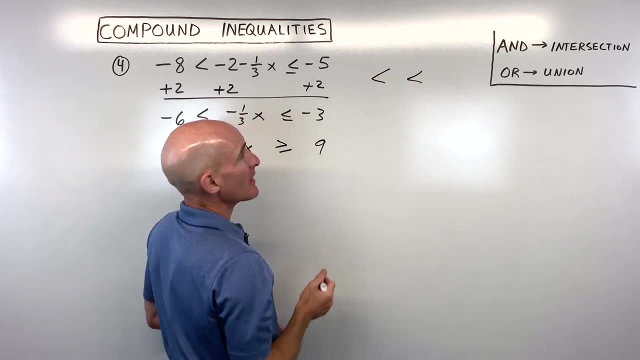 So that's going to make this a greater than or equal to. That's going to make this a greater than. But remember that little caveat we talked about earlier: You really want these inequality signs to be pointing to the left. You want them to be less than, or less than or equal. 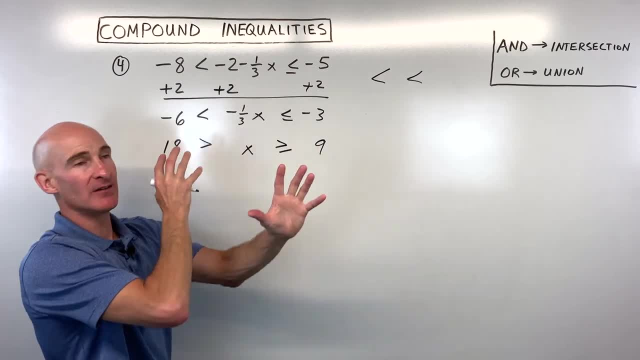 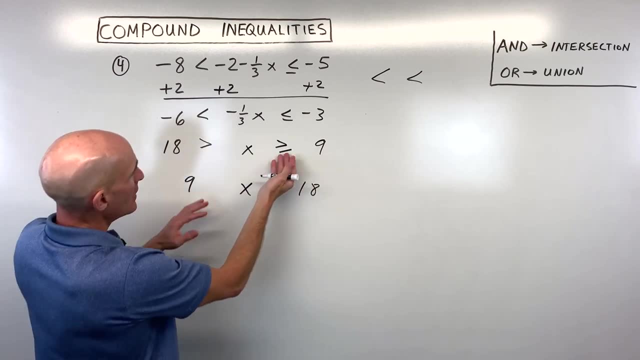 to signs. So what I have to do is pick up this whole inequality and flip it. Okay, so that's what I'm going to do. I'm going to take it, flip it over. This is going to become: 9 is here, 18 is here. When I flip it, this is going to be a less than or equal to, And. 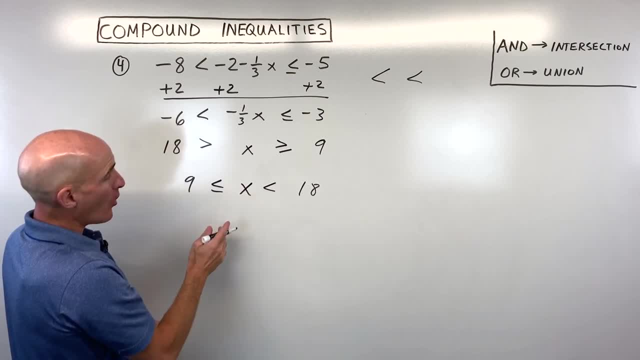 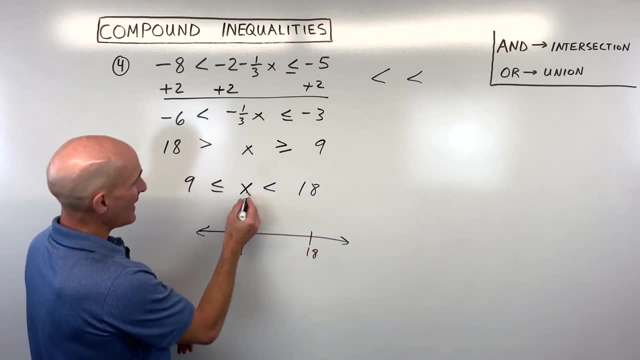 this is going to be a less than Now. it's going to be a little bit easier to graph. We can go on our number line. We can say: here's 9,, here's 18.. And x is sandwiched in between 9 and 18. It's actually greater than or equal to 9.. See greater than or equal to 9.. And 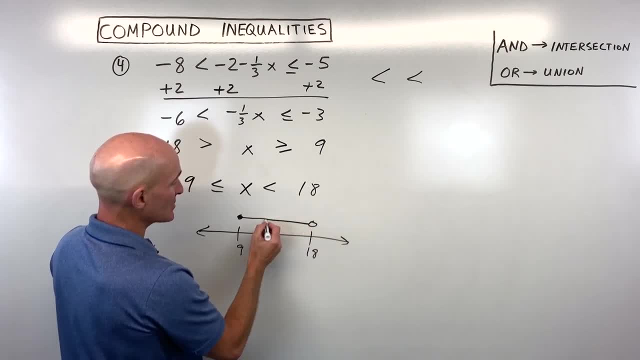 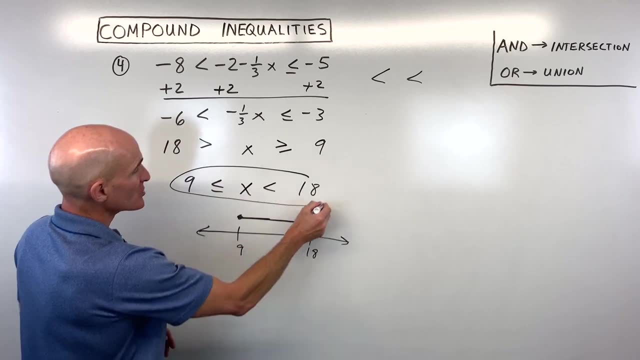 at the same time, it's less than, or smaller than 18.. So it's in between 9 and 18.. It includes 9,, but it doesn't include 18.. So this is, you know, your solution. This is like a grand. 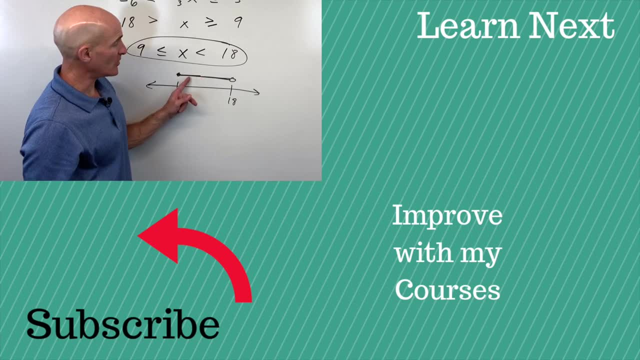 graph of our solution. And remember this includes not just integer values but fractions and decimals and basically everything in between these two points. So great job if you're able to follow this video. If you want more practice, I'll put another video right there. Follow. me over to that video and we'll get some more practice. I'll see you there.